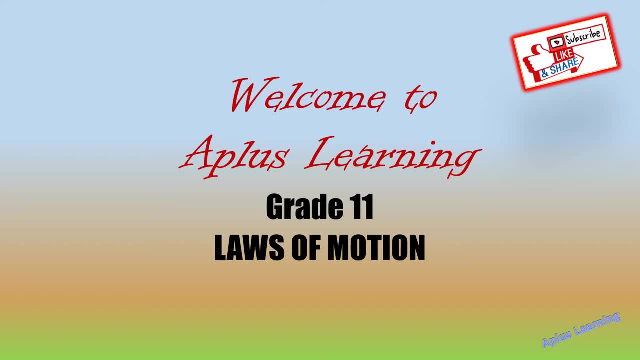 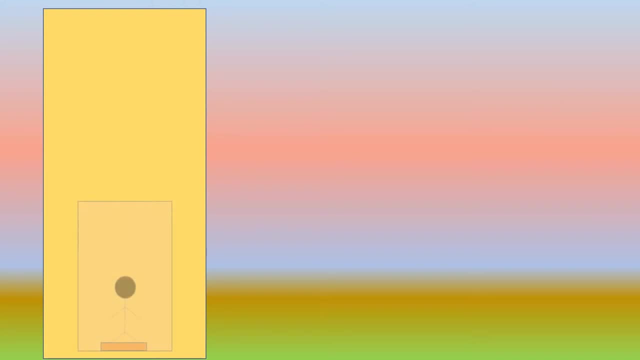 Hi, children, today we will be doing the topic of elevator physics from the chapter loss of motion. Today we will be learning of how we feel when we are in a lift or an elevator. The topic is apparent weight in a lift, or it is also called an elevator. Now, before we go into the topic, 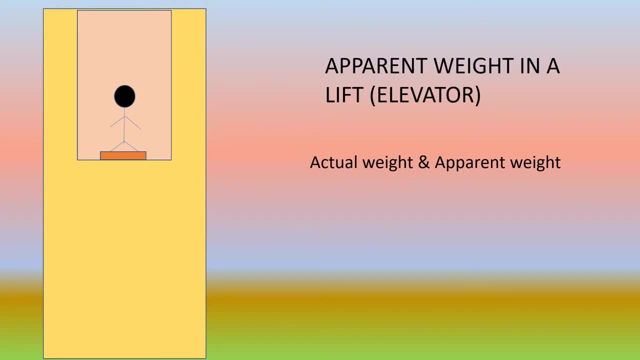 let us see what is this actual weight and apparent weight. Actual weight: we all know that what it is, isn't it, children? It is the weight due to the action of force of gravity alone. That means what weight we feel in our body, that is, mass into gravity, mass and gravity. 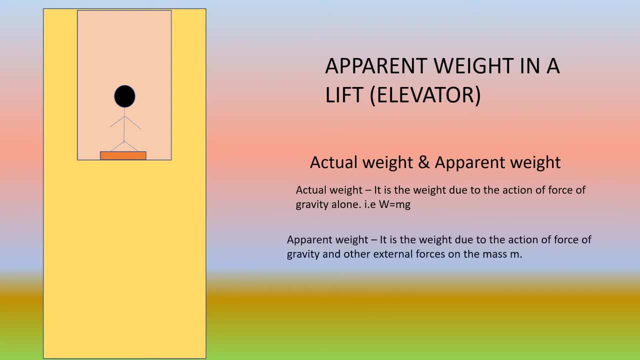 the product of mass and gravity. Now what is apparent weight? Apparent weight is actually the number of weight that we feel when we are in a lift or an elevator. Now what is apparent weight? Normal force from the scale or what is the force experienced on the body from the flow. Now what is? 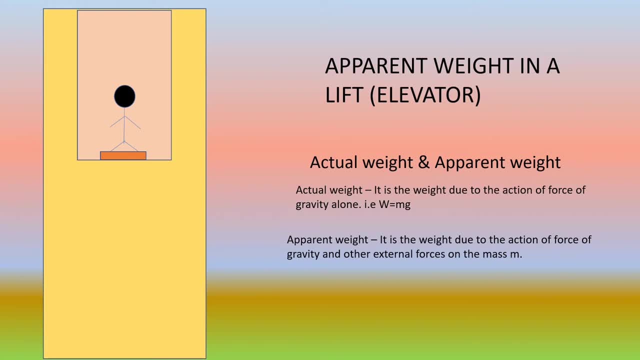 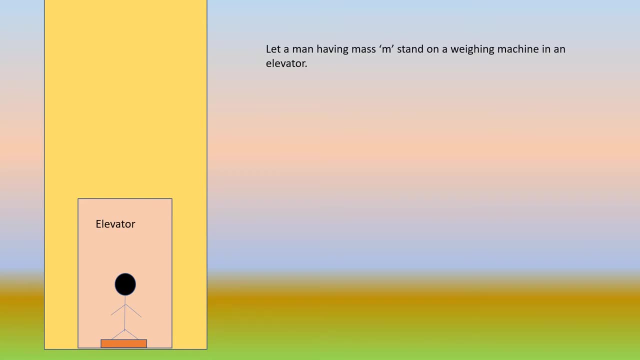 the weight due to the action of force of gravity and other external forces on the mass m. Now let's see an example of a man having mass m standing on a weighing machine in an elevator. Here the man has a mass m and is standing on the weighing scale in an elevator. Now the actual weight of the man. 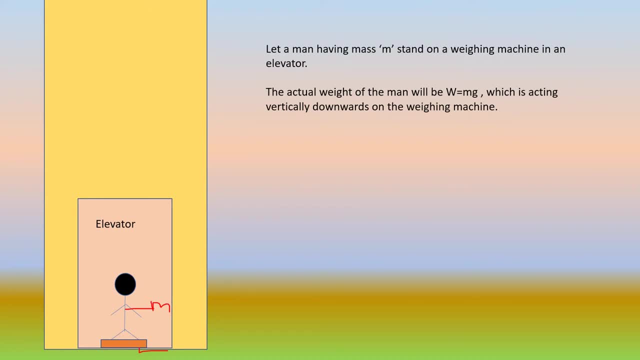 will be mg, which is acting vertically downwards. It will be acting vertically downwards and the weight will be mg. This will offer a reaction force, R, which is displayed on the weighing machine. Whatever weight is displayed, here we have the reaction force that is R, which is displayed on the weighing machine. So the apparent weight of the man is R. 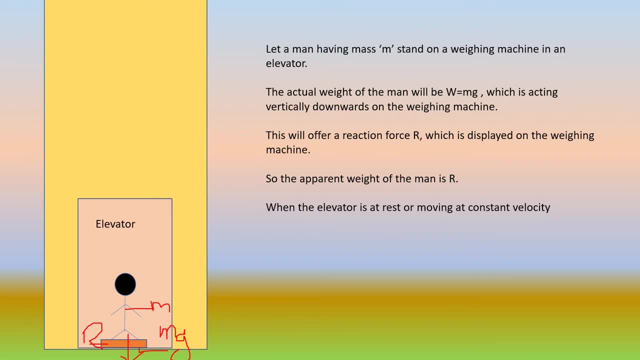 When the elevator is at rest or moving at constant velocity, R is equal to mg. This is if the elevator is at rest or moving at constant velocity. When the elevator has an upward acceleration, R will be equal to mg plus ma in solution, Whereas when the elevator has a downward, 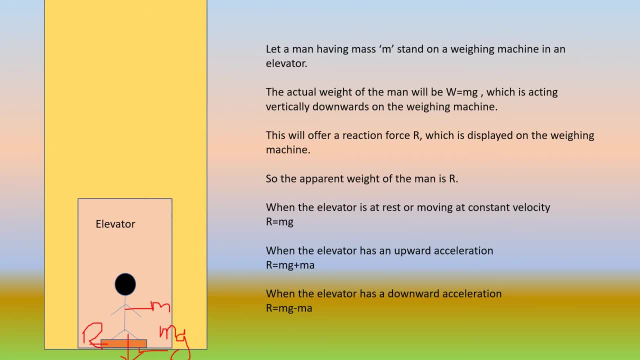 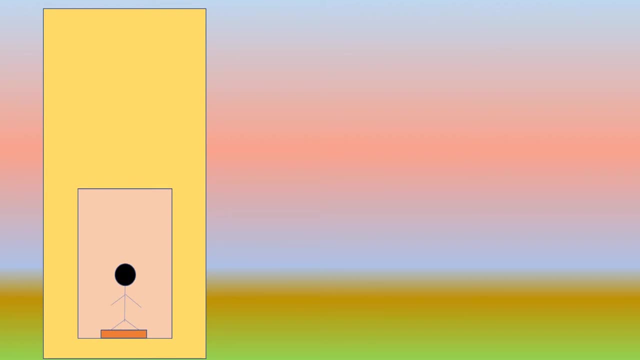 acceleration R is equal to mg minus ma. So today let us see all these in detail. Now let us see what happens to a weight when we move upwards with an acceleration. in an elevator, when the lift moves upwards with acceleration a, the net upward force on the manners r minus mg. 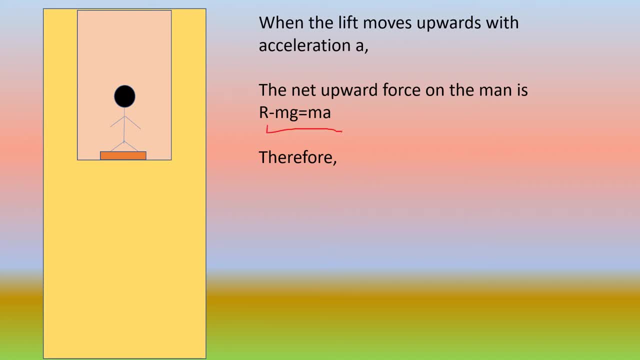 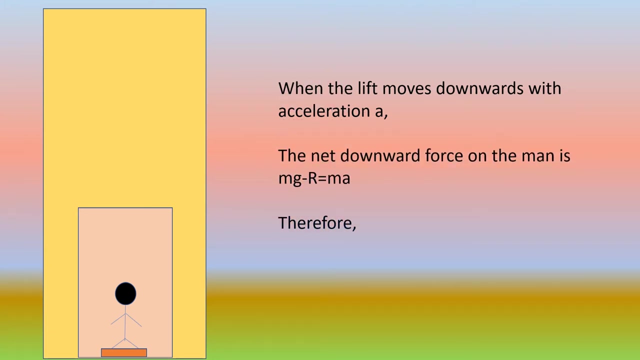 is equal to m a. therefore, the apparent weight will be: r is equal to mg plus m a. now, when the lift moves downwards with acceleration a, the net downward force on the man will be mg minus r is equal to m a. that is the apparent weight is equal to r is equal to mg minus m a. take on onto the right side and m a comes. 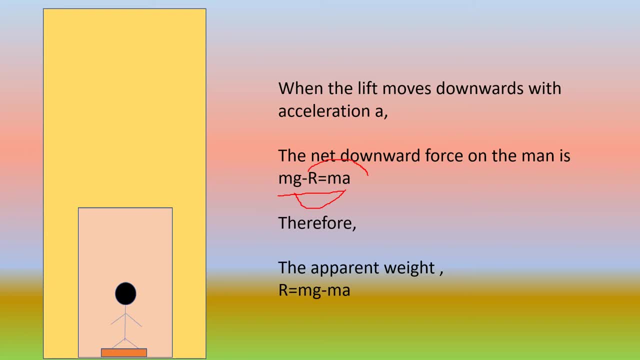 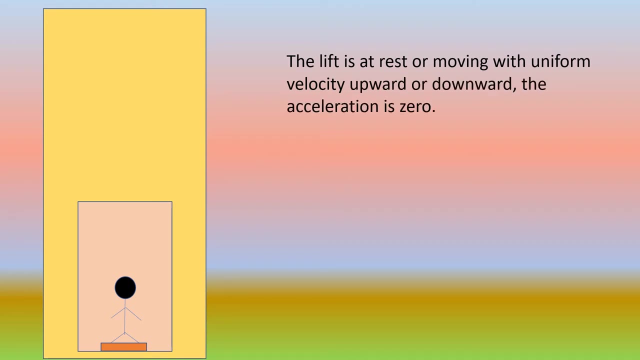 over here to the left of equal to, we get r is equal to mg minus m a. now let's see what we feel when we are in the lift and the lift is at rest or moving with uniform velocity upward or downward, when it is moving with an uniform velocity. 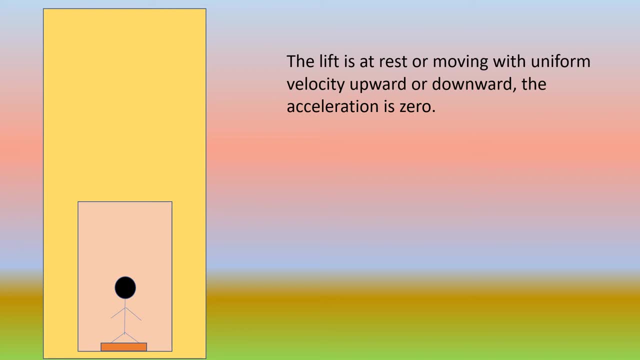 or if the lift is at rest, the acceleration is always 0, so the net force on the man is also 0. therefore, that apparent weight will be equal to the actual weight. That means R will be equal to mg. Now let's see when the cable breaks and the lift just hurtles down. When this happens, 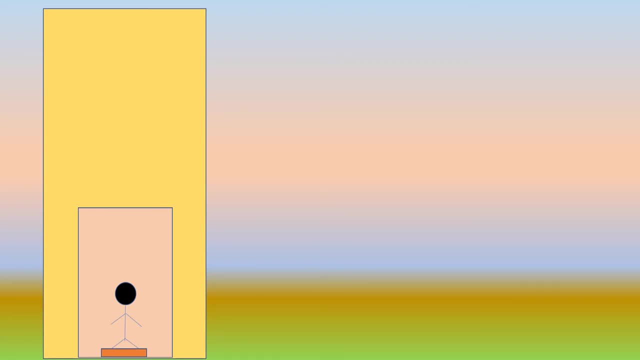 the person inside the elevator experience a free fall, And when a free fall happens, the body is entirely under the influence of the gravitation. So when the lift falls freely, the body weighs zero on the weighing machine, but its actual weight is still mg.